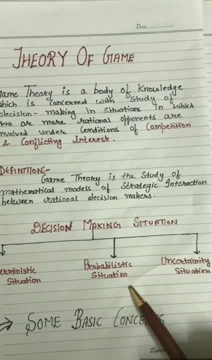 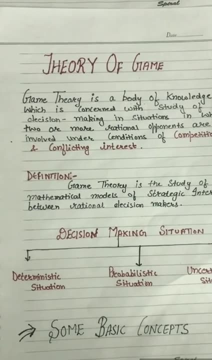 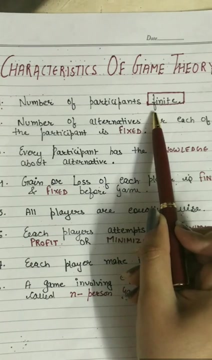 First one is deterministic situation, Then probabilistic situation And then uncertainty situation. Before studying concept of game theory, first understand what are the characteristics of game theory. First characteristics: number of participants is finite. What does it mean? Whenever we play a game, we decide from the beginning that the number of participants 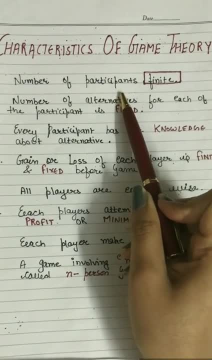 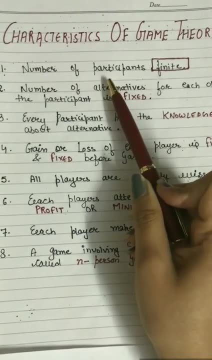 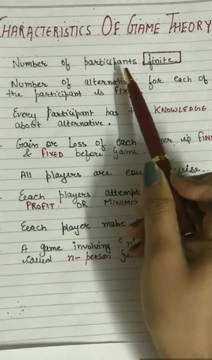 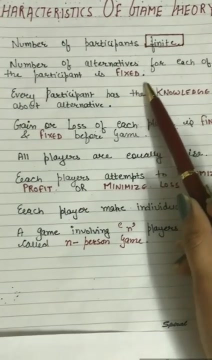 is finite. So if the number of participants is finite, then we decide that there will be four players, six players. If we lose, then we add 2 more players in order to win the game. It means number of participants is finite. Before starting the game, we have to decide how many players. 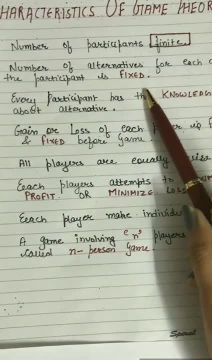 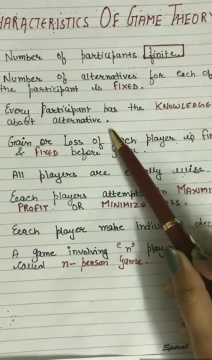 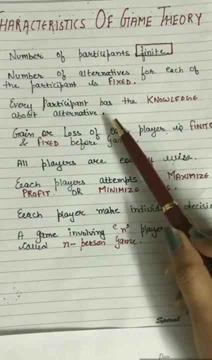 will play that game. Second, characteristic number of alternatives for each of the participants is fixed. The rules are already fixed in game. We cannot change the rules And that is why we will come to the 3. Every participant has the knowledge about the alternative. 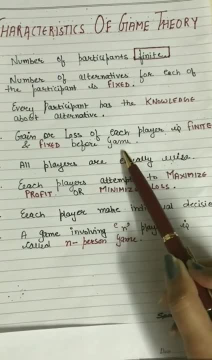 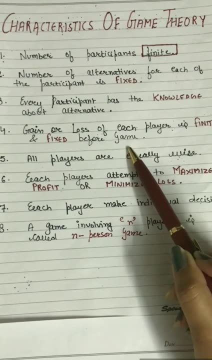 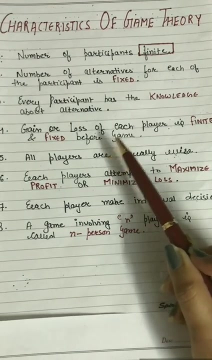 4. Gain and loss of each player is fixed, and fixed before the game. For example, if you play a game and you have decided that whoever wins will have to pay 100 rupees, So that amount has already been decided, that whoever wins the game will get 100 rupees. 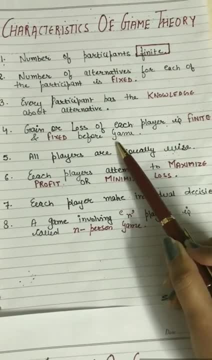 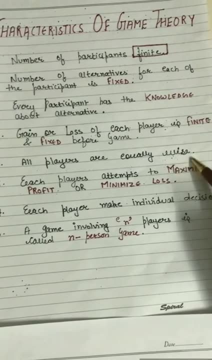 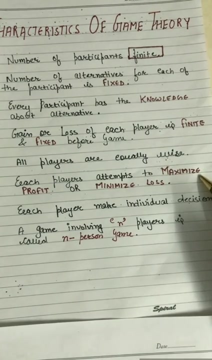 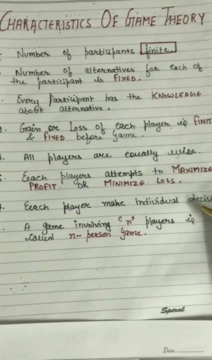 So we decide that before playing the game, that what will be the benefit to the winning player? 5. All players are equally wise. Next point: 6. Each player attempts to maximize profit. 7. Each player makes an individual decision. 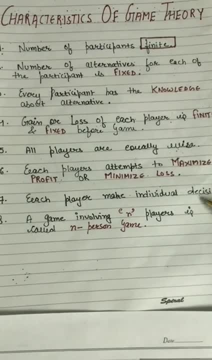 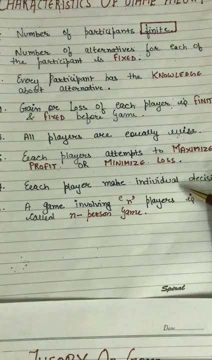 Whenever you play a game, your decision is independent. You do not take a decision by asking someone else. 8. A game involving N players is called N% game. If you play a 2% game, you will call it 2% game. 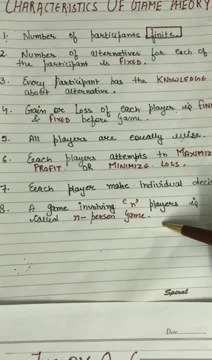 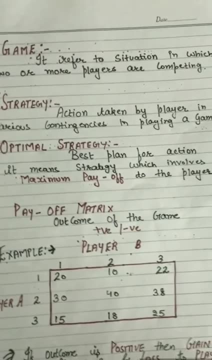 If you play a 3% game, you will call it 3% game. If you play a 4% game, you will call it 4% game. This is all about the characteristic of game theory. Now moving towards some basic concept of game theory. 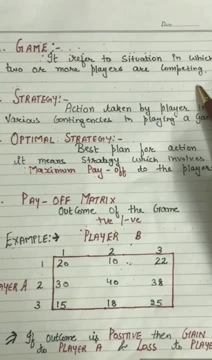 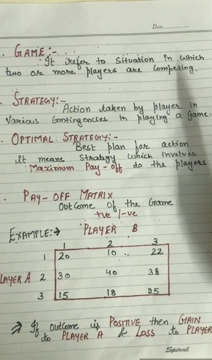 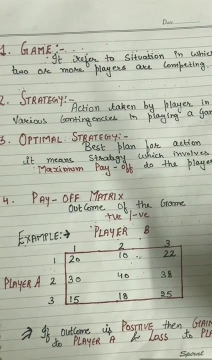 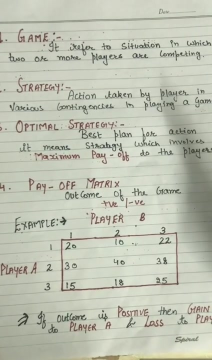 1. Game: Game is a situation where two or more players are competing with each other. For example, IPL Students are competing to take the first position. So these are all other examples of game. 2. Stratygy: 3. Stratygy is the strategy that an action player is taking to win. 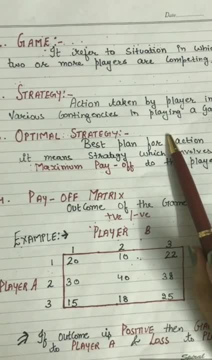 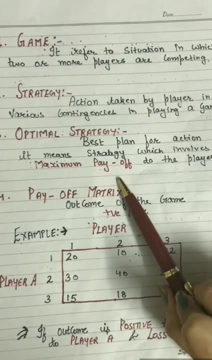 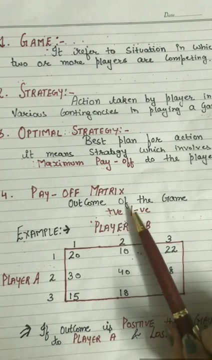 4. Optimal strategy. Stratygy can be more than one. Optimal means when you are selecting the best strategy for getting maximum pay off. That is called optimal strategy. 4. Pay off matrix- matrix. Pay off matrix means the outcome of the game, the result of the game we call. 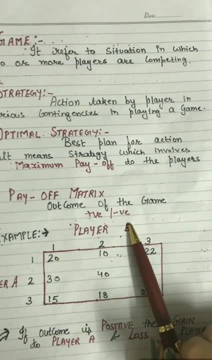 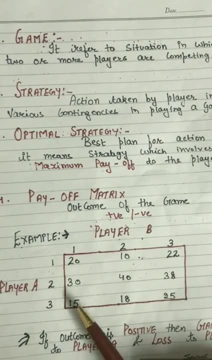 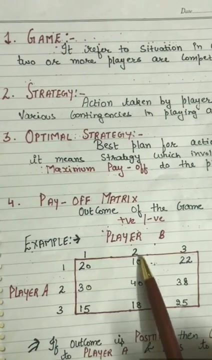 it pay off, It can be positive or it can be negative. Now we will do pay off matrix with an example. When will it be positive and when will it be negative? We are assuming there are two players in a game: player A and player B, Player B adopting three strategy: 1,, 2,. 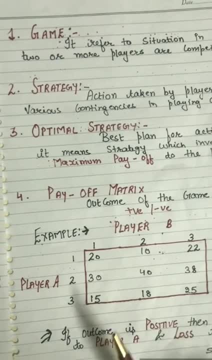 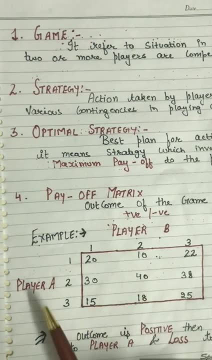 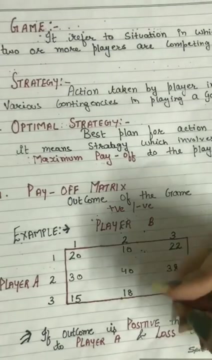 3.. Similarly, player A also has three strategy: 1, 2 and 3 strategy. In this table all outcome are positive. If all outcome are positive, then it means gain to player A and loss to player B. But if I place in this strategy minus 40, it means player A adopts second. 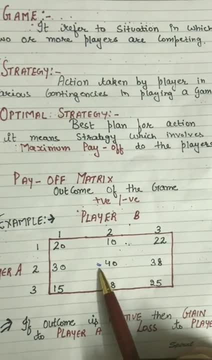 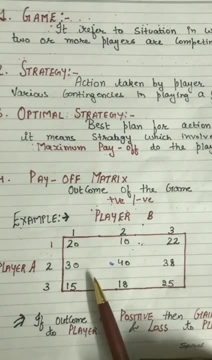 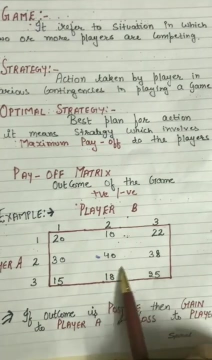 strategy. player B also adopts second strategy and it become minus 40. Then it means gain to player B. If there is all positive outcome, it means gain to A and loss to B, And if there is some negative value in pay off matrix, it means gain to player B and loss to player A. Moving 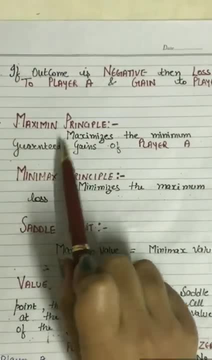 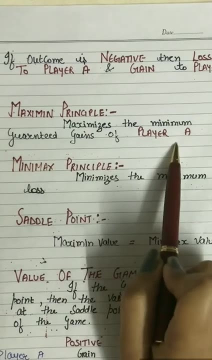 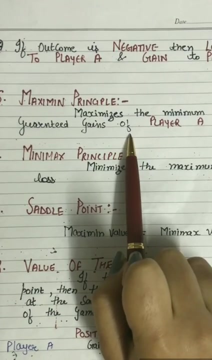 to our next concept, fifth point, that is, Maximin principle. Maximin principle means maximize the minimum guaranteed gain of player A. In this, what happens is that the gain which is going to be there, he wants to maximize it. Who wants to do it? Player A. So we call. 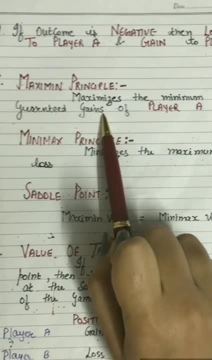 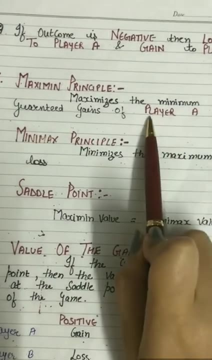 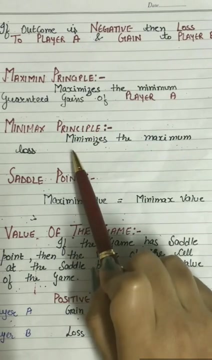 it maximize minimum gain. That is known as Maximin principle. And minimax principle means minimize the maximum loss. If player A is gaining, he wants to maximize it, And if player B is losing, he wants to minimize that loss. These are two principles which we will follow. 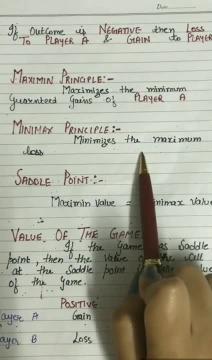 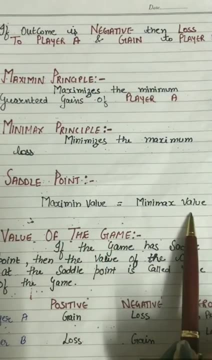 in this game theory, And we will see this in detail, along with the other two principles. So we will see this in detail, along with the other two principles. So we will see this in detail, along with the problem. Now, next point, seventh point: saddle point, Where maximum value is equal to minimax value. 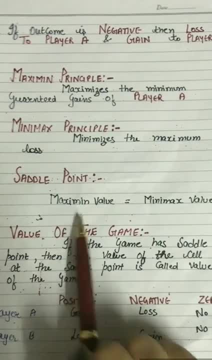 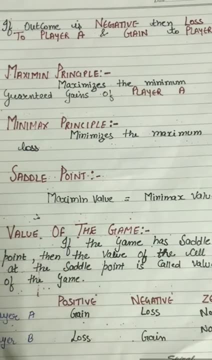 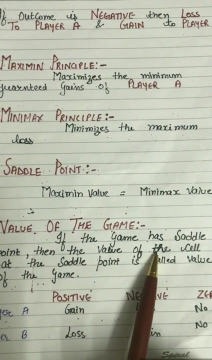 that is saddle point. Where our maximum value is equal to minimax, it means the gain of player A is equal to the loss of player B. that point we will call saddle point. Eight value of the game. If a game gets a saddle point, then the value of the sell at the sale. 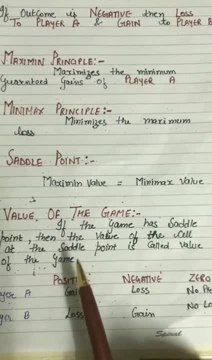 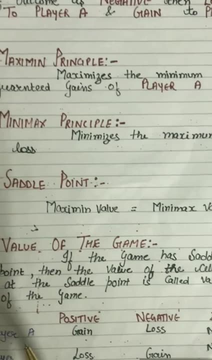 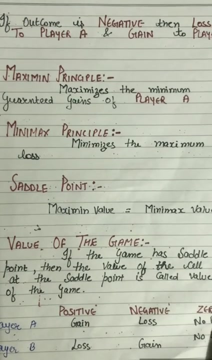 point is called value of game. And suppose what gain A gets Regional value 8.. And what loss belongs to: B also goes for 8.. So eight is the value of the game, Minimum A gained, and Comme A isn't there, Value of the game can also be positive, negative, zero, Positive. 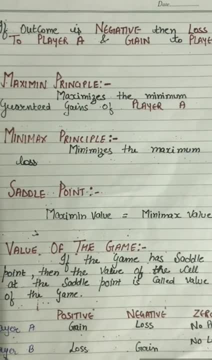 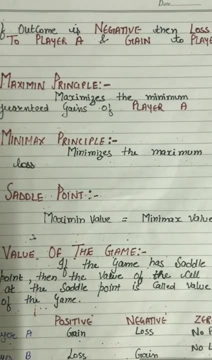 player A gainedyg Negative player B loss. time WE TURN TO MINIMUS. And how negative was the player B? Negative player A gain 紅, then player B will gain and when there is positive value, then player A will gain. 0 means no profit. 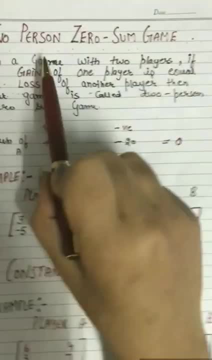 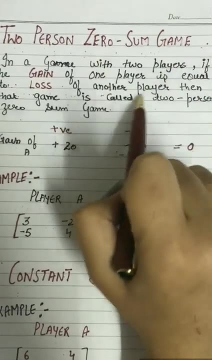 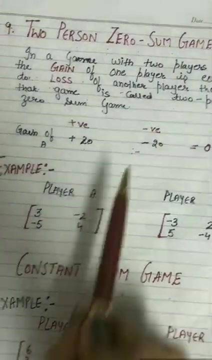 or no loss situation. next concept, 9th concept: 2%, 0 sum game. now we have said in the character set that there is n% game because we are talking about 2% of player A and player B. so that game is 2% and we have used 0 sum game. what does 0 sum game mean? that the gain of 1 player 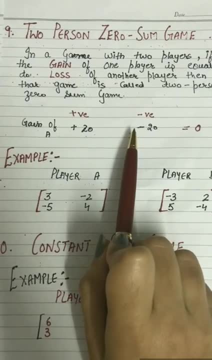 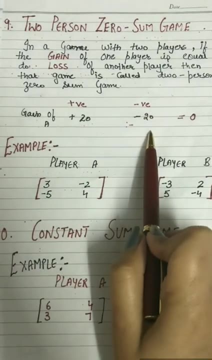 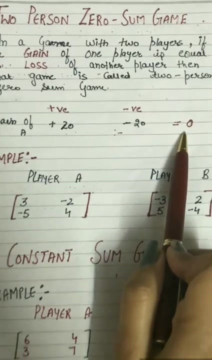 will be equal to the loss of 2 players. so we will call that game 0 2% game. suppose, if A gained 20, then this game lost 20, so its value will be 0. that is why it is known as 0 sum game. we are doing this from the starting: A gain and B loss. if A is gaining 20 and B 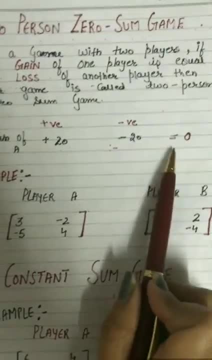 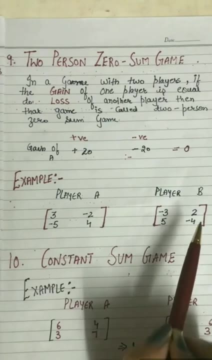 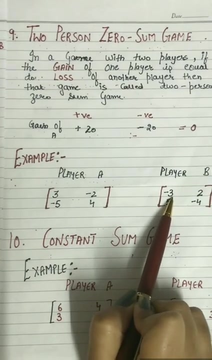 is losing 20, so if we do sum on, then we will get that sum 0, what we call that 0 sum game. take an example: player A, player B. if player A adopts this strategy, then it is gaining 3 and player B is losing its corresponding minus 3, but sum will be 0 minus 2. it means 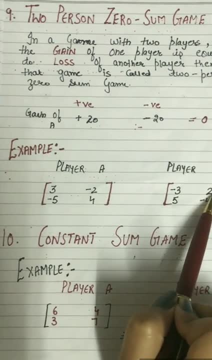 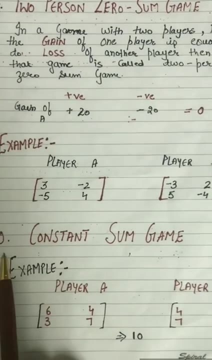 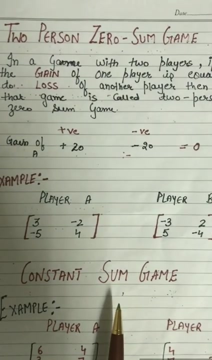 player A is losing and its corresponding player B is gaining 2 again, sum will be 0. that is known as 0% game. moving towards next concept, 10th constant sum game: we have said above that 0 sum game, gain of 1 and loss of 2 when it is equal to 0. that 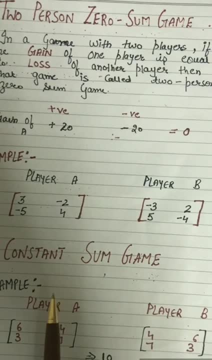 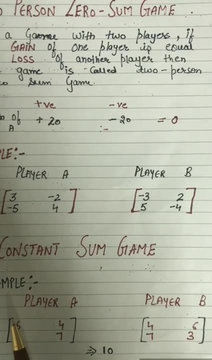 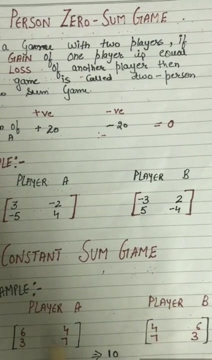 is known as 0 sum game. what happens in constant sum game? that the gain of player A and the loss of player B will not be 0. we will get a constant value. take an example: player A gained 6 and player B is losing 4. so if we are gaining 4, so 6 plus 4 is 10. player A is 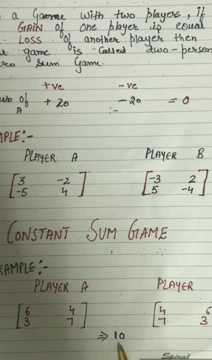 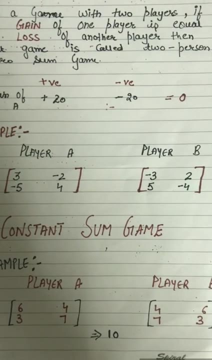 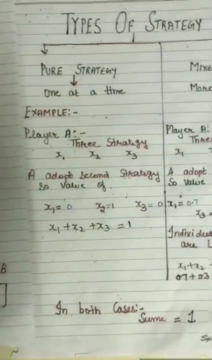 losing 6 again, sum will get 10. this is known as constant sum game. this is all about concept of game theory. now, second, what are the type of strategies? strategies are the course of action which are choose by the competitor to win the game, and always they will try to. 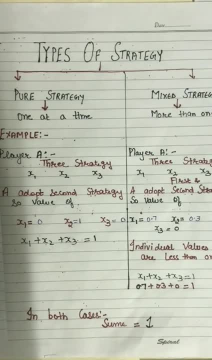 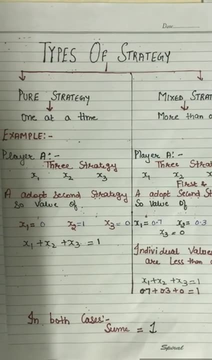 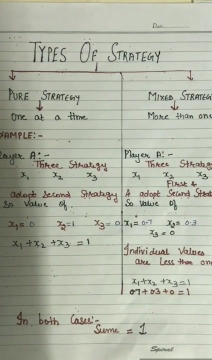 find the optimal strategy. optimal means best strategy. there are two type of strategy. first one is pure strategy and second is mixed strategy. first one is pure strategy and second is mixed strategy. when we talk about pure strategy, it means player are following one strategy at a time. at a time, they are following only one strategy. and when we talk about mixed 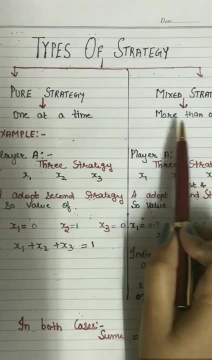 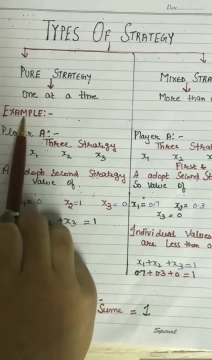 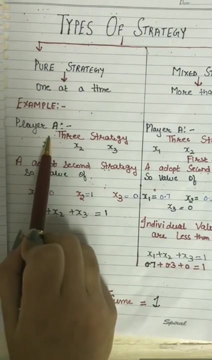 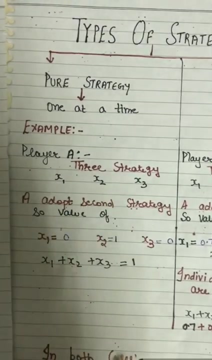 strategy, then what the player is doing. they are following more than one strategy. let us take understand with an example about. first, we will talk about pure strategy, when player is adopting only one strategy at a time. for example, player A has 3 strategies and player B has 3 strategies: X1, X2 and X3. A is adopting second strategy, so when A is adopting second. 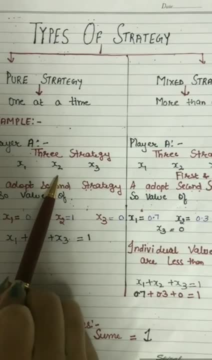 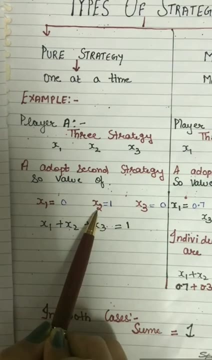 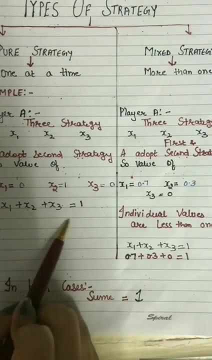 strategy because it is pure strategy. then at a time there will be only one strategy. then value of X1 is equal to 0, X3 is equal to 0 and X2 the strategy which he adopted. its value will be 1. so when we will plus their payoff then we will get that value equal to 1 always. 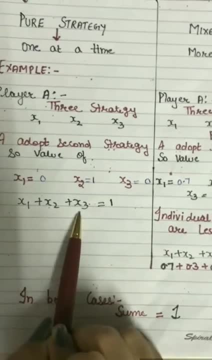 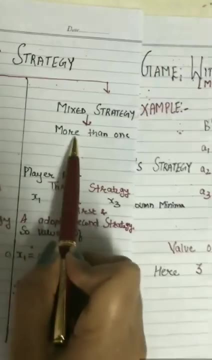 so every time when we will summer the payoff, thenин the payoff of 25 X 1, X, 2 X 3, their sum will be equal to 1. moving on the next strategy, that is, mixed strategy. in this case, player adopt more than one strategy at a time. pure strategy in mix: very more, more strategy. 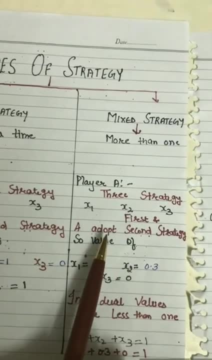 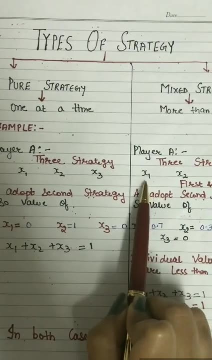 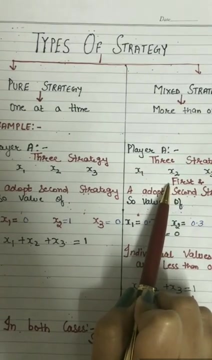 have adopted. for example, player A had adopted 2 strategies- one is X 1 strategy and one is X 2 strategy, and probability value in this one will be less than one in X 1- X 2 strategy, But the sum of all three strategies will always be equal to 1.. 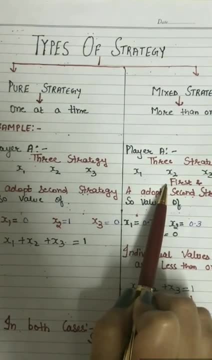 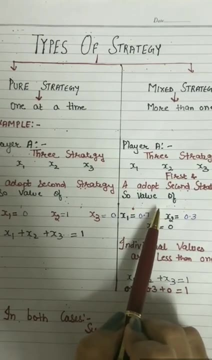 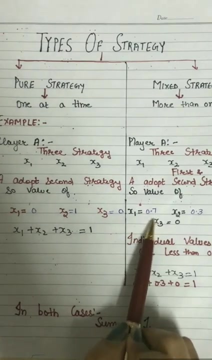 In pure strategy, the values other than the strategy adopted were 0.. But in mixed strategy, the value of the strategy adopted will be less than 1.. But their sum will always be 1.. If X1 is adopting the strategy, then it is 0.7.. 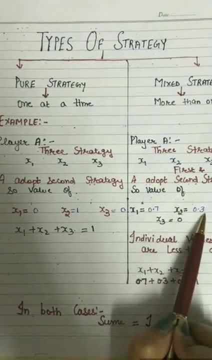 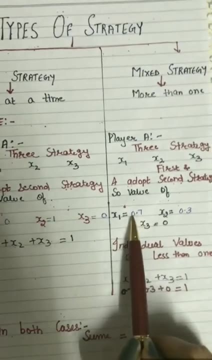 If X2 is adopting the strategy, then it is 0.3.. Both the values are less than 1.. If X3 is adopting the strategy, then the value is 0. Because it is not adopting X3. It is adopting only two strategies: X1 and X2.. 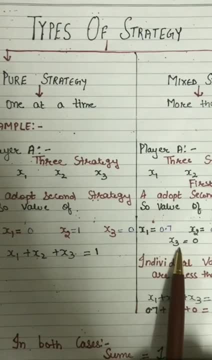 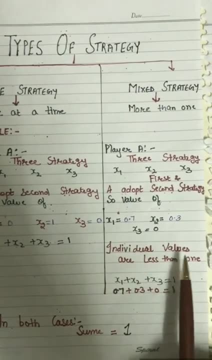 So the value of the remaining strategies will be 0.. The strategy you will adopt will have only that value, And the value of the other strategies will be 0.. If we look at their individual values, then they are less than 1.. 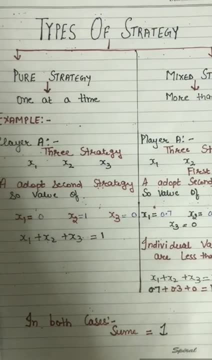 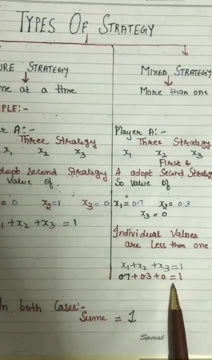 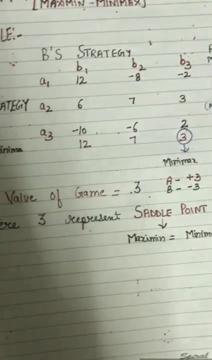 But if we do their sum, then it is equal to 1.. So in both the cases the sum of their payoff should come, Whether it is pure strategy or mixed strategy. Now we will start the game with pure strategy. We will discuss pure strategy with an example. 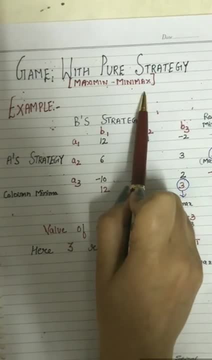 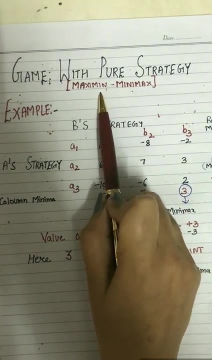 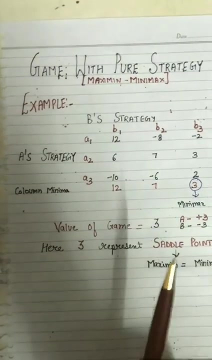 This is also called Maximum Minimax Strategy. What strategy is this? Maximum Minimax Strategy Means what we have to do in this. We have to maximize the gain of A. We have to minimize the loss of B. Now we have to find the optimal solution. 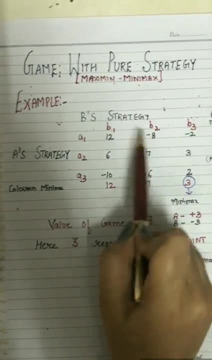 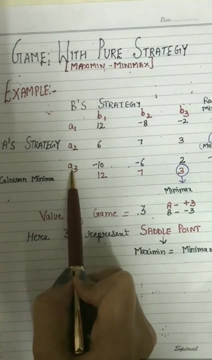 Here you have a question. B is adopting three strategies: B1,, B2, B3.. The player A also has three strategies: A1,, A2, and A3.. What is your first step? First, you have to find the minimum value of the row. 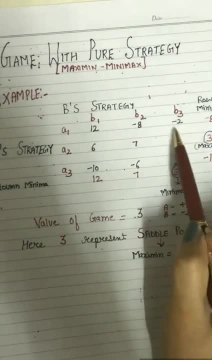 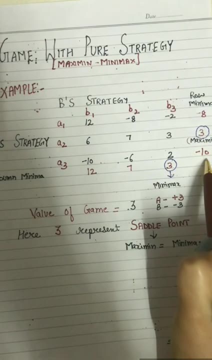 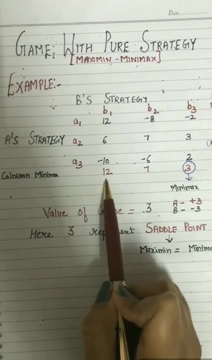 Means the minimum value of the row. So what is the minimum value of this row Minus 8.? What is the minimum value of this 3.? What is the minimum value of this Minus 10.? Second step: we have to count the column maxima. 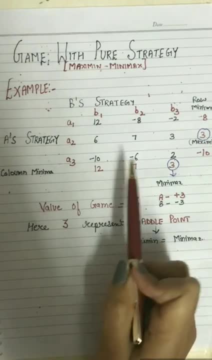 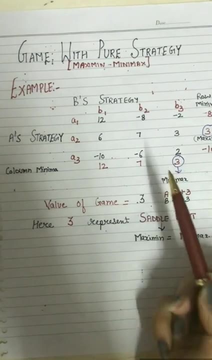 So what is the maximum value of the column 12.? What is the maximum value of this 7.? And what is the maximum value of the third column 3. When we took out the row minima and the column maxima, 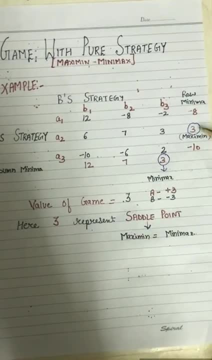 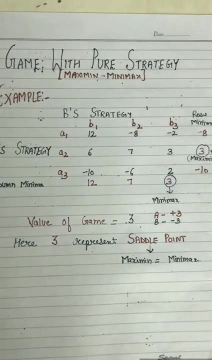 after that, what is our step? Take the maximum value of the row minima. Why are we doing this? Because A wants to maximize his gain. So here we assume that if A wants to maximize his gain, then the maximum value is 3.. 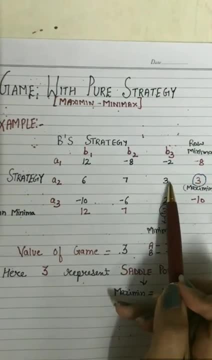 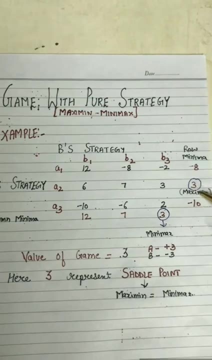 Which strategy should A take? A2,, B3. And at the same time, if we talk about B's strategy, then we have the minimum value of B. If A wants to maximize 3, then B wants to reduce the loss of 3.. 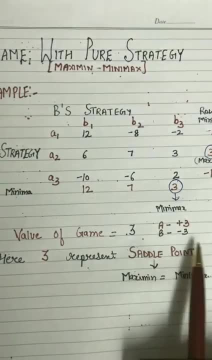 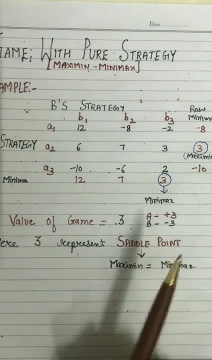 So this 3 is the same in both. Therefore the maximum value of B and B is called value of gain. That is, if A gets a 3 again, then it is plus 3.. If B loses 3,, then it is minus 3.. 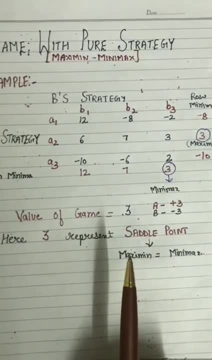 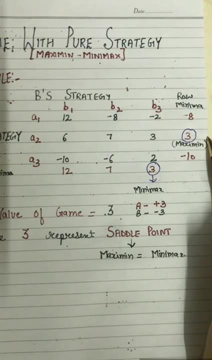 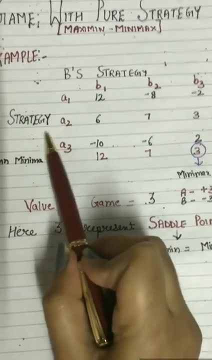 And when our maximum value is equal to minimax, then we call it saddle point. So what does this 3 represent? Saddle point? Now there is the confusion that children have a lot of thoughts that Here we will get the minimum and here we will get the maximum.